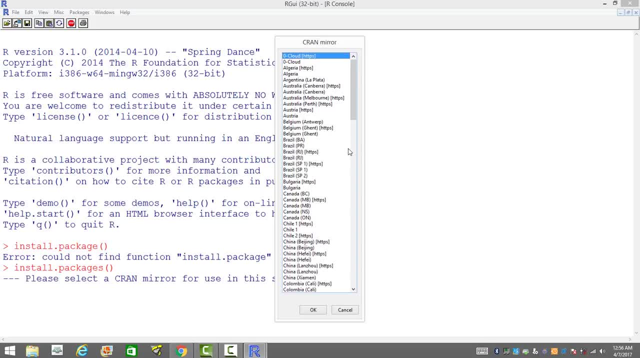 You should go ahead with selecting the one that is very closest to you. So, since I'm in UK, so I can, you know, choose something from one from UK. So I can choose Cambridge, London, So I'll go with Cambridge. 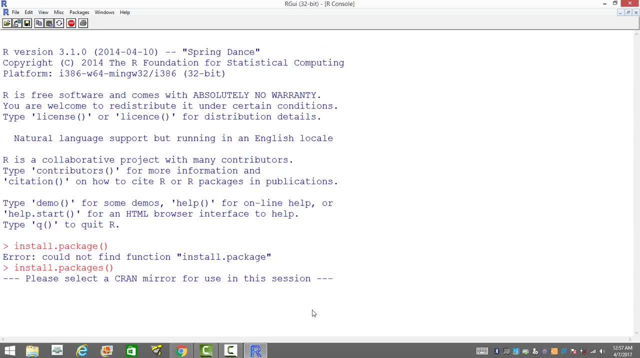 So once we have, you know, selected the location of the server from where we want to install the package, the next prompt that is going to show it to us is the packages names. Okay, So now that we have the list of packages, you know, it's in order, sorted in order. So we can, you know, we can just find it out that which, which package do we want to want? and there's so many of them, over 5000, that's what, that's what I know, and it is increasing, ever increasing with time, because many people are contributing towards. 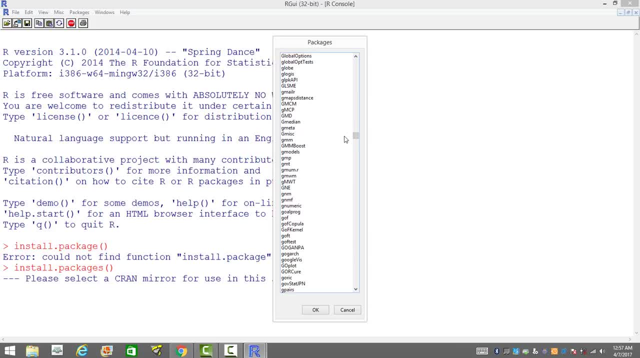 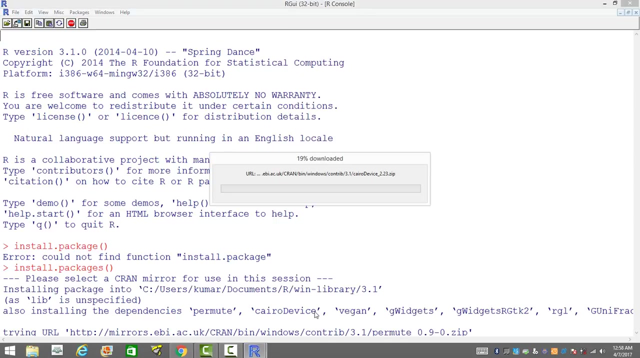 the, our open source libraries. so let's, let's install any of this package. we can, you know, let's install G quad. all right, okay, maybe you can install grammar, okay, so we just select that and just press ok and it is going to install. now you can. 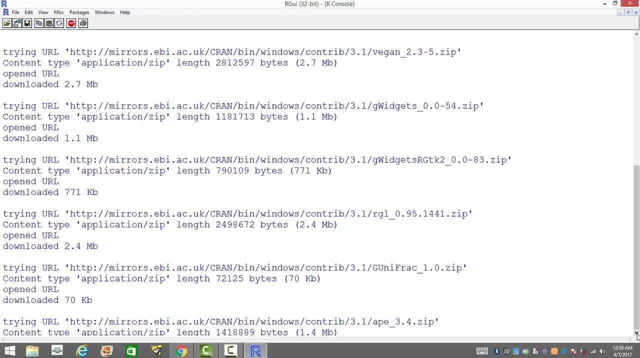 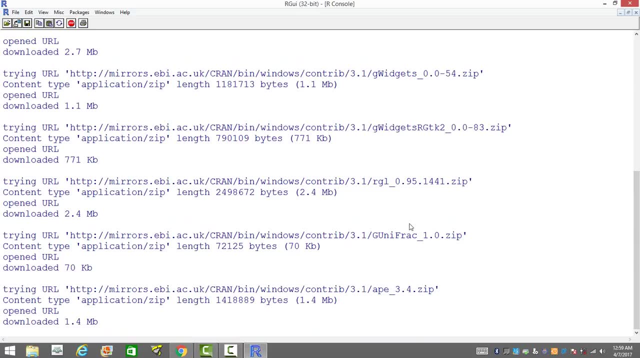 install, you just have to. so what it is doing is that it is. it is downloading from the. you know the firm's clan. many of this, many of these packages which got downloaded are from grant, which is the official place where you know you can download our and our packages. so that's the. 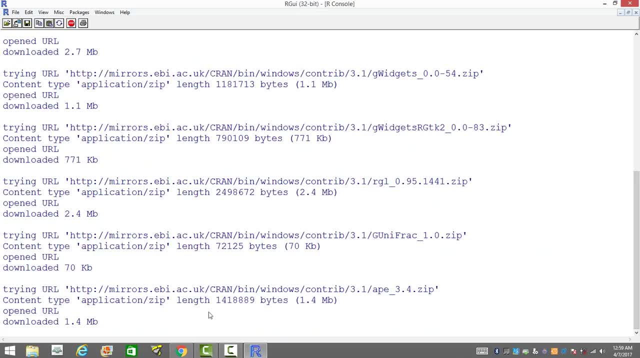 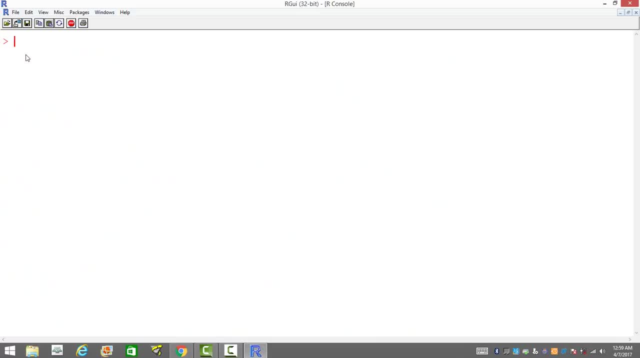 website where you can, you can find. okay, it's still the case. okay, now that the download process is over, you can load the package that you have, that you have just, you know, installed. okay, so for that you just have to write library. and then what is that? G? 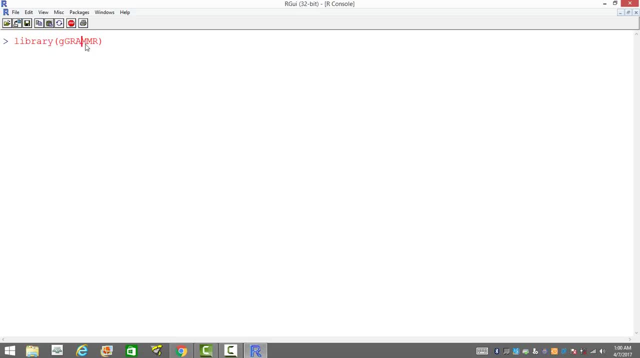 so library, and then provide the name of the package and that's going to. you know, uh install for you. okay, so I have another uh package I have already installed, so I'll just show you to go gz plot to. I've just installed, so when I uh go to load it, yeah, so now it's it. 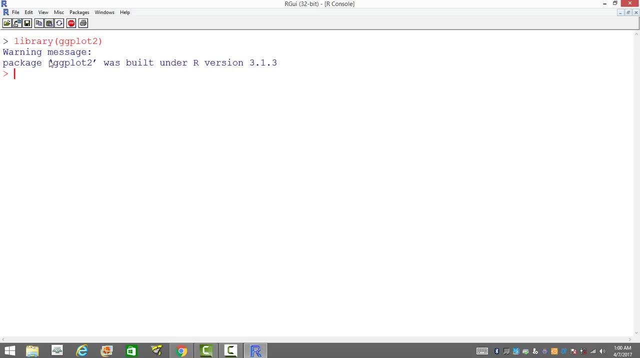 got loaded uh onto a sas, on your, onto your r session. now you can use it. uh, you know for for gplot. you can use it to plot your data. um, if you want to get more help about installation, you just have to type in help and then packages. 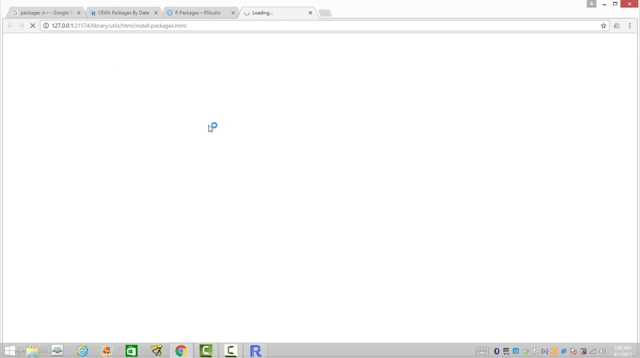 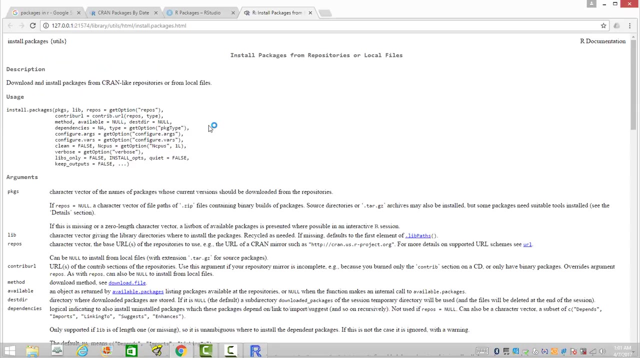 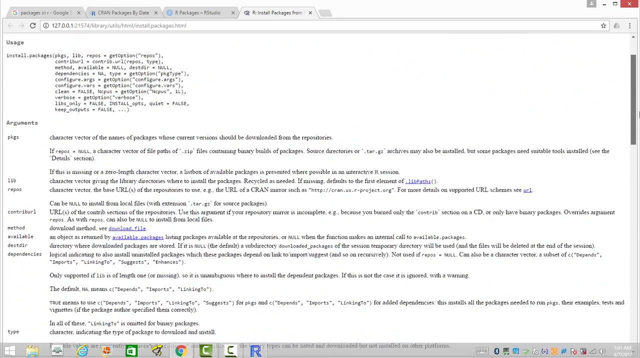 okay, okay, now it is going to take you to the internet and you will get, um you know, different uh informations about loading uh our packages, um. so if you want to learn more about it, so there is a page dedicated on the cran website. you can read it thoroughly to get more information about how to 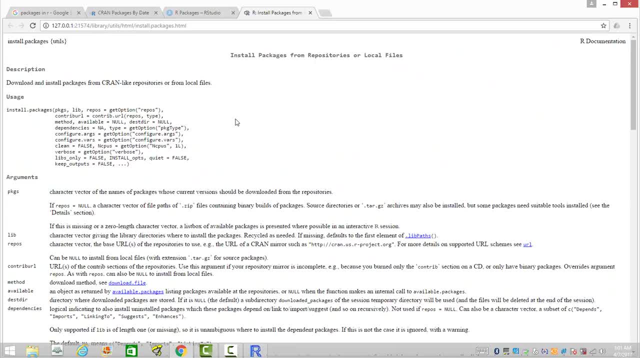 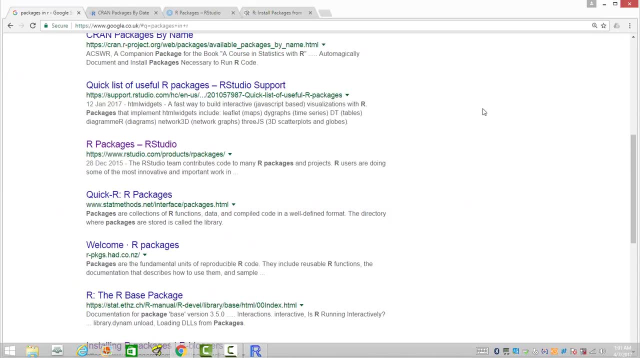 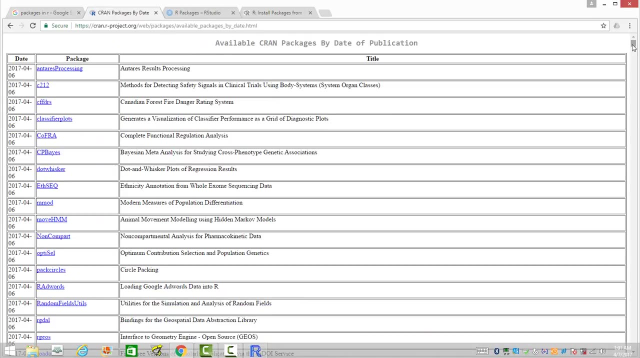 you know, load packages in different forms. all right, so if you want to know what are the different packages available uh in our, just you know type in packages in our- in the first uh url itself, uh, you will find the cran website where it has got the list of packages available to you and 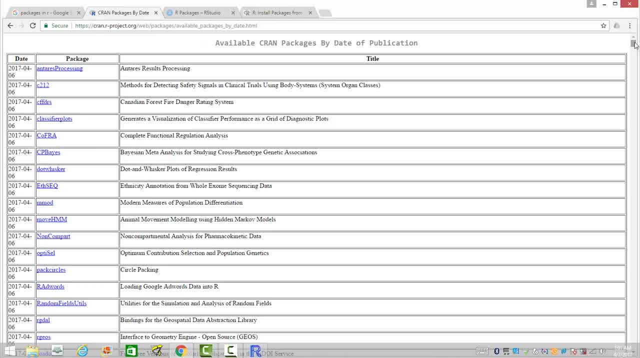 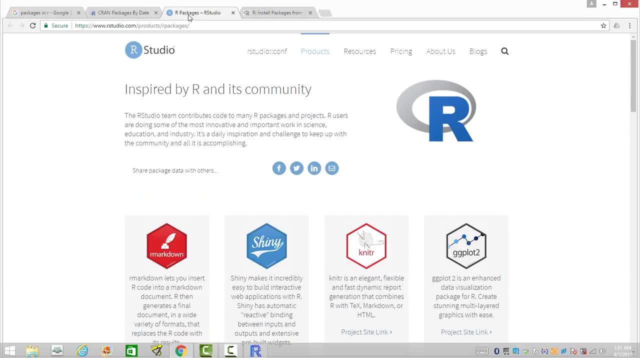 you can just select as per your, you know, requirement. so the description of each one of these packages, what exactly a particular package does, is given, uh, in this list. um, all right, and you can also get many of these packages in our studio for using our studio, then this is where. 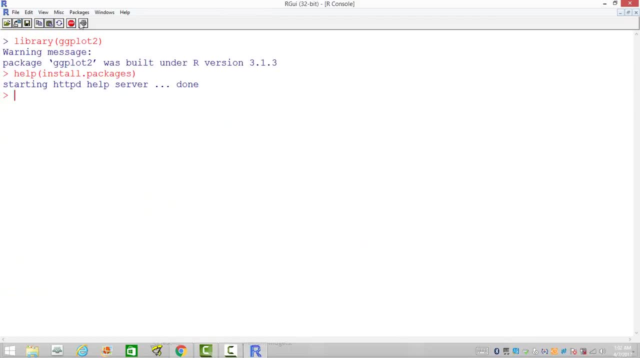 you can get the details of the packages. second way of doing it is uh using the menu bar. so we have got package. so first you you need to do what uh is, just installation of package. so that's the first step. so when you try to install a package, 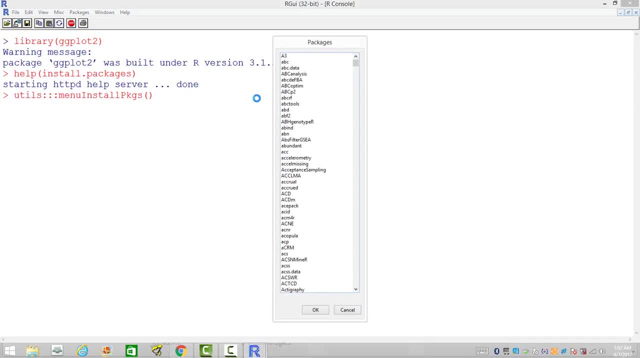 it's going to again do the same. it will ask us, uh, to choose the server, given that we have already selected the server from where we want to download the packages, that's not going to prompt again, but, uh, otherwise it is going to prompt you, you know, and uh select.